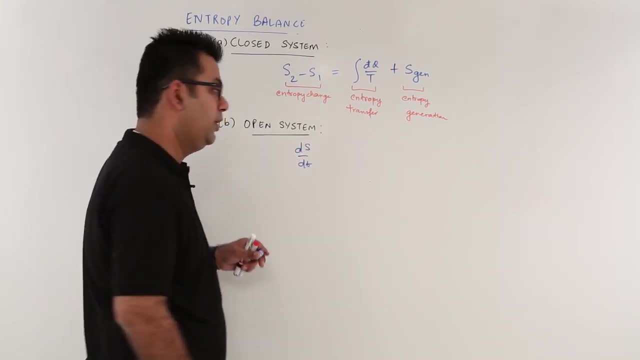 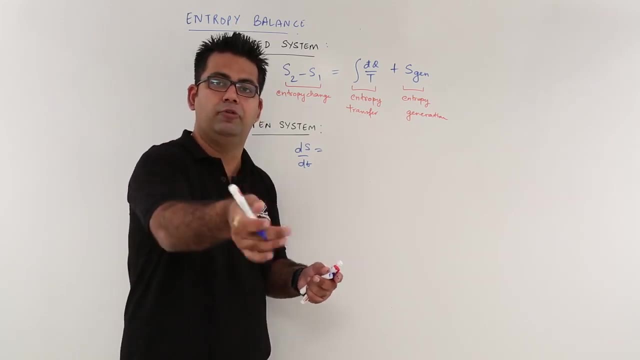 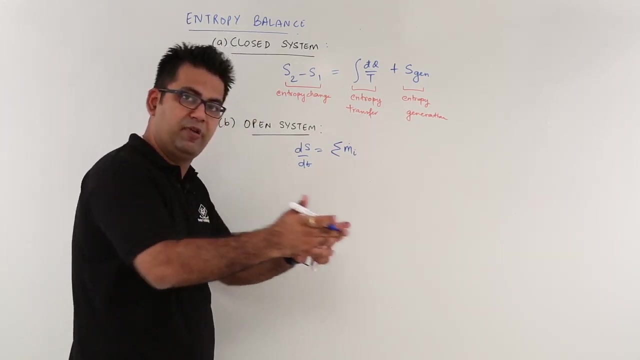 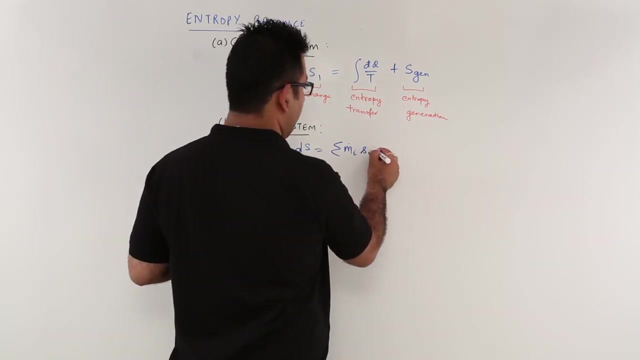 Okay, That is the rate of change of entropy. This is a sum of the net entropy transfer due to the mass inflow and outflow. So you will have the mass inflow rate. You can have multiple streams coming in into the entropy that comes in with it, minus m. 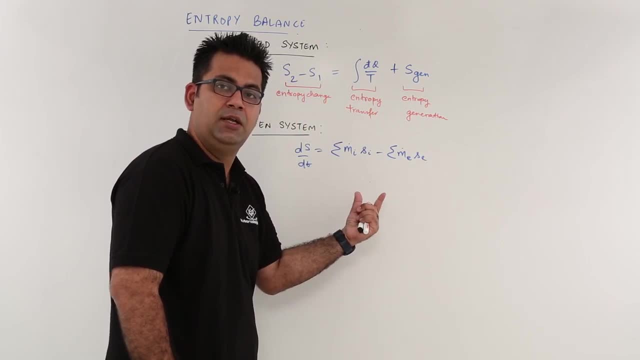 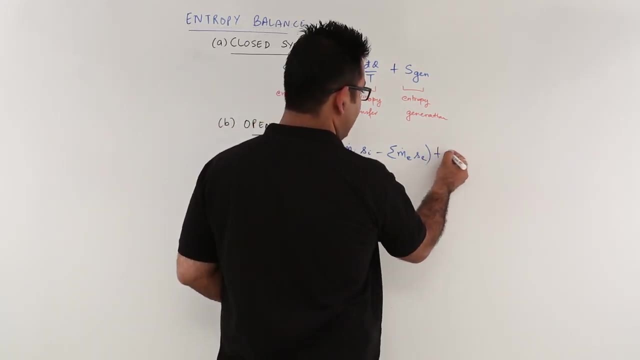 e into S e. So this is the net entropy change rate. Okay, So this is the net entropy change due to the mass inflow and outflow. Okay, This is one part Plus. yes, we have some entropy transfer due to the- you can say- heat transfer across the. 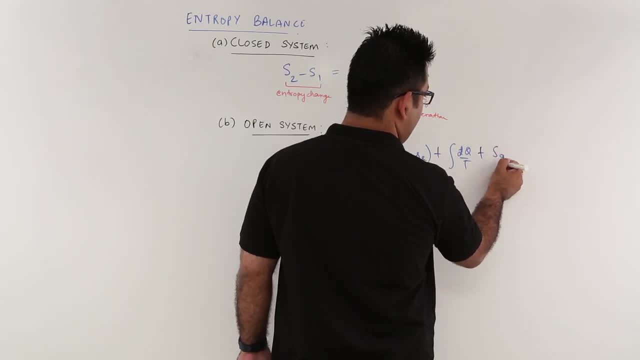 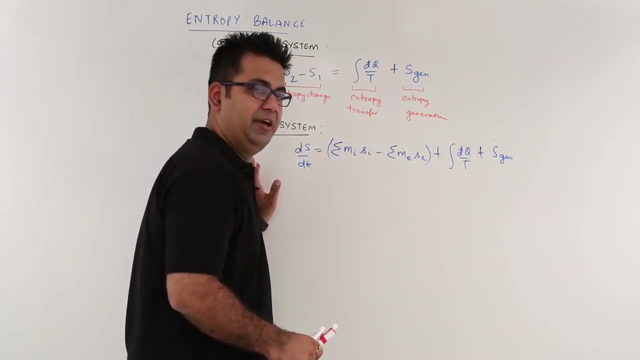 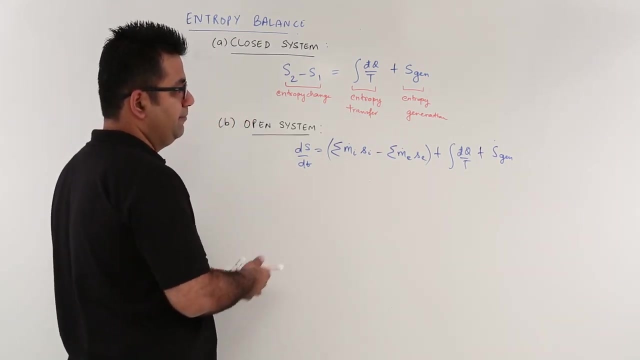 boundary, Okay. Plus, there will be some heat generation within the system. So this is quite different from the closed system equation. So this is something you need to understand. Okay Now, if your you can say equation or your process is adiabatic. 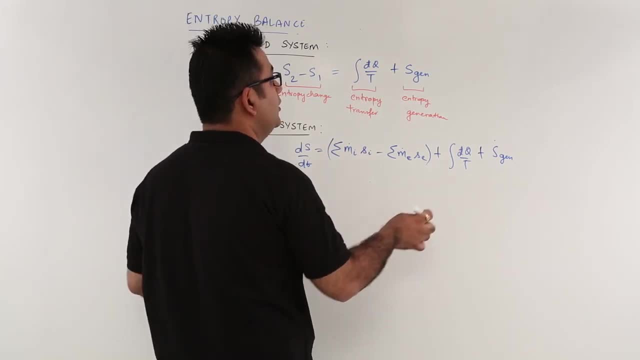 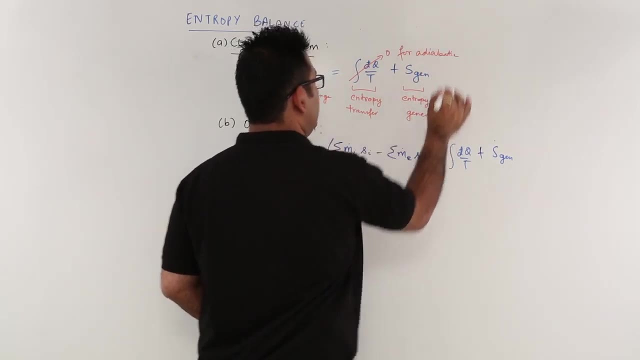 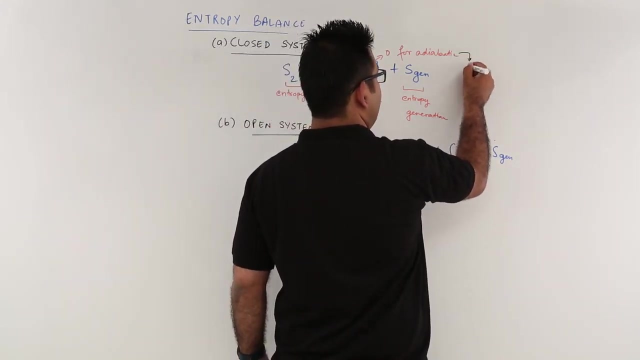 Okay, So in this also, if you have your adiabatic equation, So this would become 0 for an adiabatic process. Okay, So for an adiabatic process this would become 0, and then we can say that for adiabatic delta. 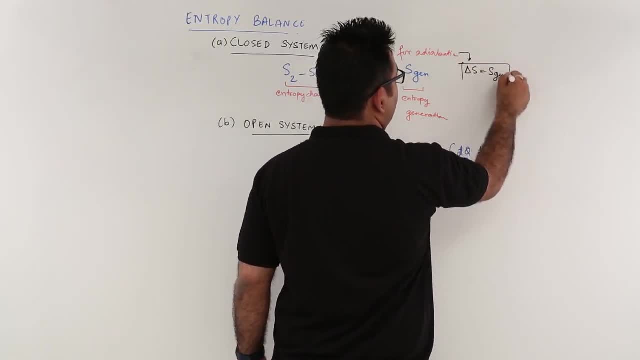 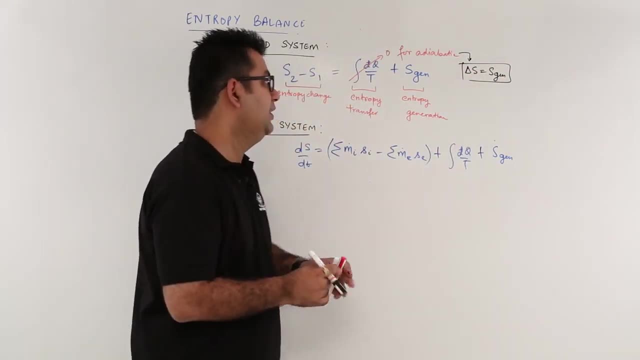 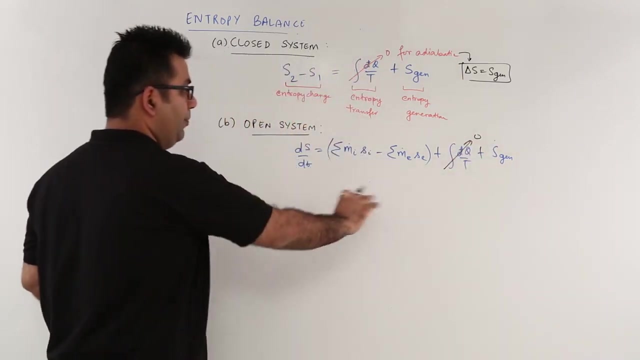 S is equal to the entropy which is generated. So whatever generation of entropy is there, that would be the change of entropy in the whole process, and that is only true for an adiabatic process. If you put this 0 in the open system, then you would have ds by dt is equal to. I can. 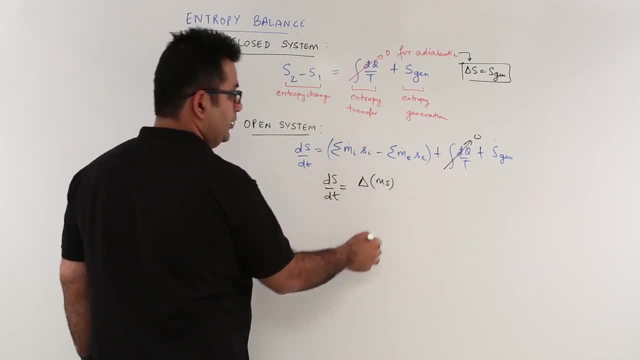 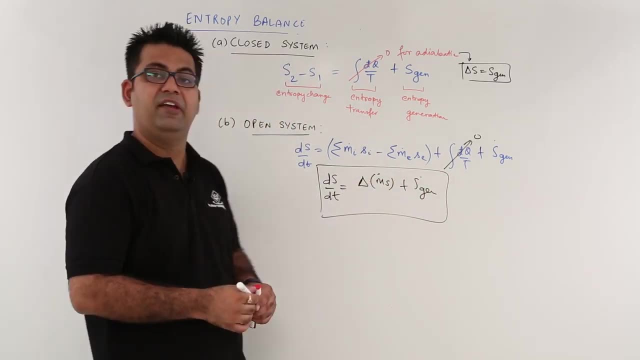 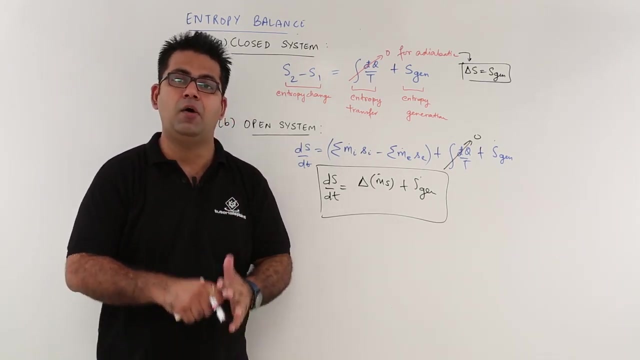 say, delta of ms plus whatever heat generation that you have. Okay, So these two formulas are very, very important for you to remember and understand for entropy balance in a closed and an open system respectively. Now, in the next video onwards, we will look at some questions on entropy and you can say: 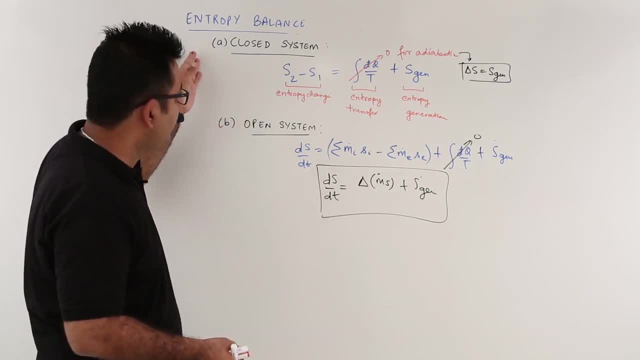 which are the applications of entropy balance on a closed system and an open system. So now let us move on to the question solving on the chapter of entropy. Okay,